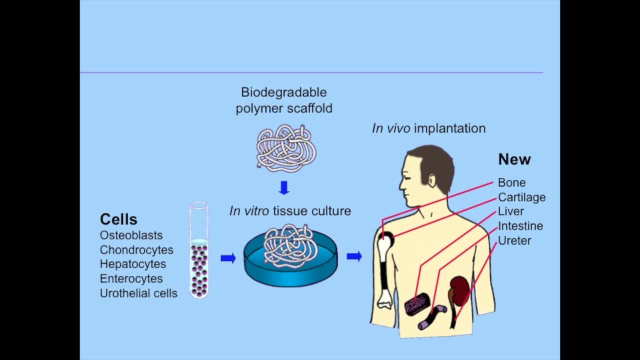 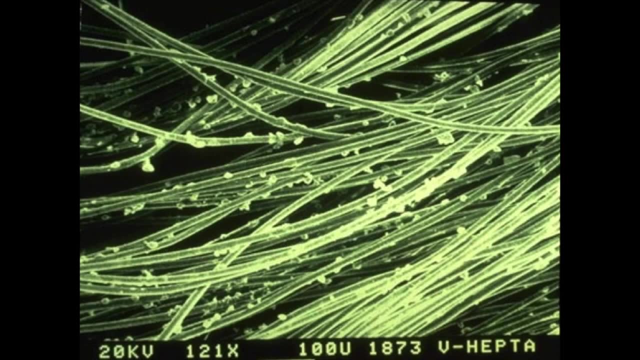 culture. You have to have the right stresses and so forth to actually make them grow in the right way, And then you could make the tissue. Just to show you a few pictures, we converted these into scaffolds where you'd have fibers and cells. And Prasad Chastri, who was one of my postdocs. he now runs a big institute in. 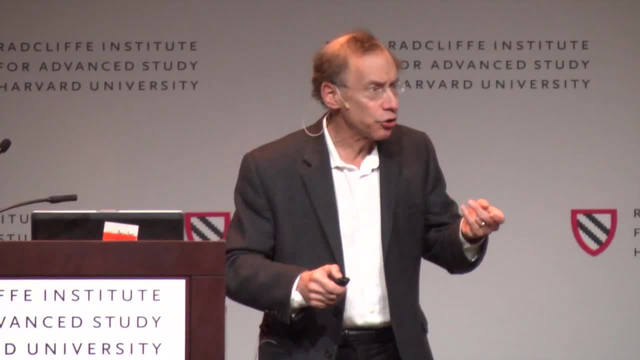 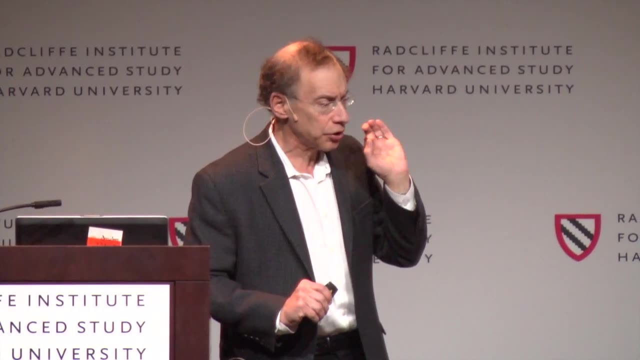 Germany. he actually worked out a way, using CAD-CAM techniques like computer-aided design, to make these into virtually any shape, And then you could use things like three-dimensional printing or various foam techniques to make these into different kinds of forms. So let me just give. 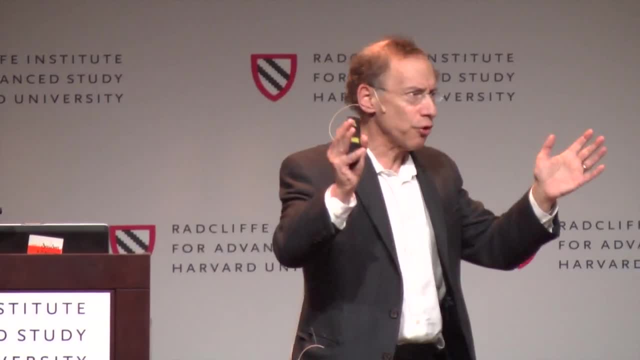 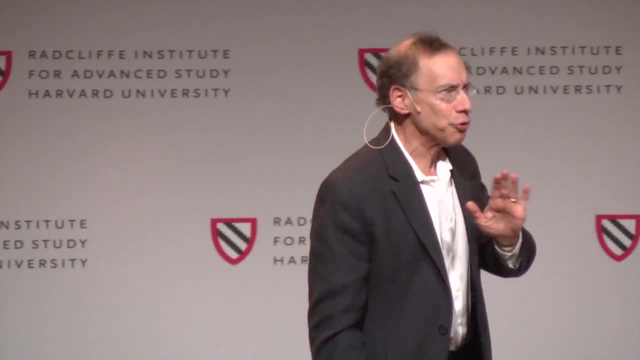 you an example, And this is pure speculation. but let's say, 30 or 40 years from now, somebody comes to a plastic surgeon and they say: we want a new nose. So my speculation is that there'll be a computer screen and you'll have a. you can look at the screen and you can have your choice of 40 different noses. 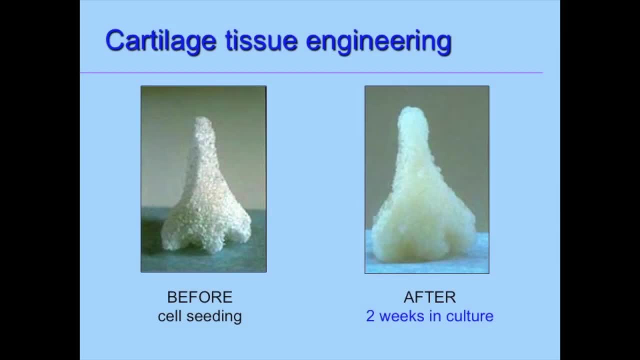 any shape. And to that end, what Prasad did is he worked out ways to make those noses. They're actually three-dimensional, 98% porous, but you could take cartilage cells from the patient themselves- I'll give an example shortly- and make the nose. 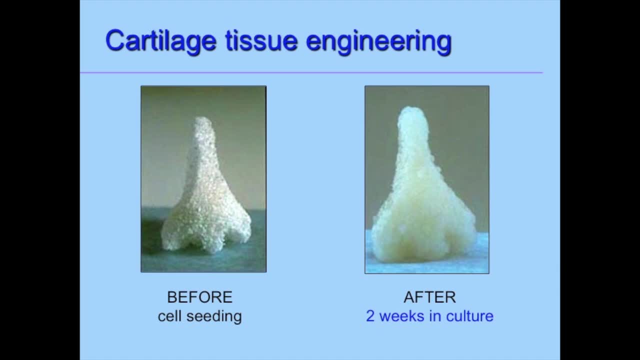 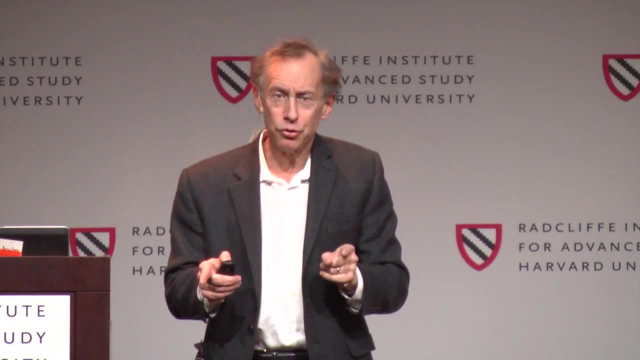 Now this is kind of like a regular nose. But let's say, somebody wants an upturned nose. Well, you just take a little bit of this off. that's not so hard to do. What if somebody wanted a hooked nose? I mean they. 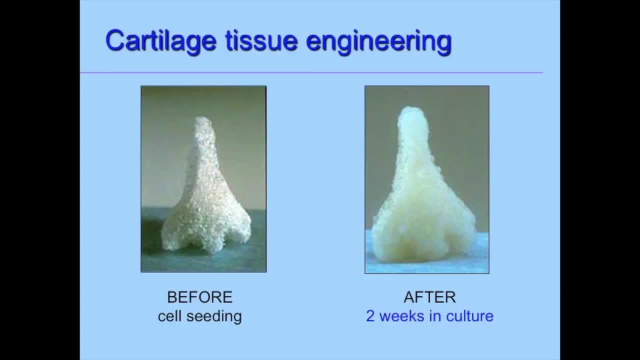 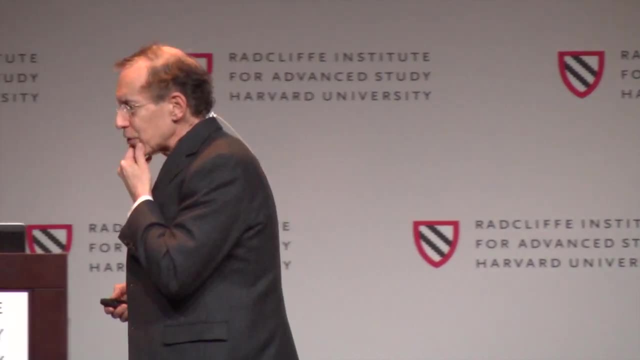 probably wouldn't, But if they did, we'd just give them a little bit more, So you can really do these any way you wantTo this end, I'll give you a couple of examples: Chuck Veconte- Chuck actually was in the newspaper today- worked with us, And Chuck actually was the one- was the two people who just first came out of that población crisis and became a professor is work with us. I don't have the ceremony right now, but I'd say their CNC had to come out the next day and was going to work with us and become part of the upturned nose. 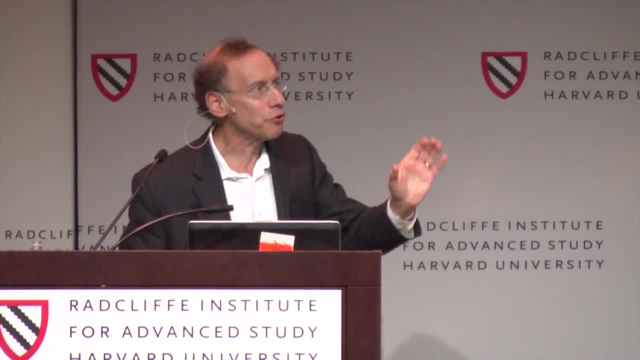 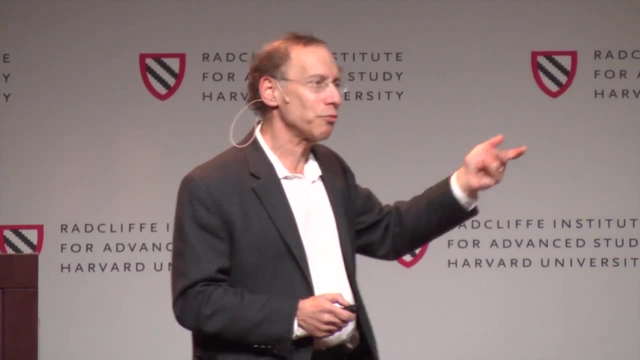 was the one with the two people who just had the discovery of how you could give acid to convert certain cells to stem cells. But now we go back to the 1980s, when he'd get started working with Jay and myself and one of the things he did was make new cartilage. 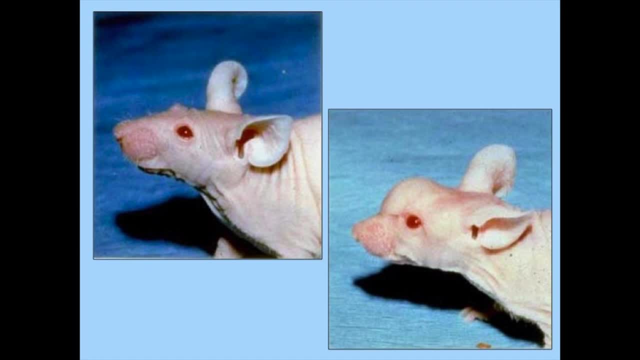 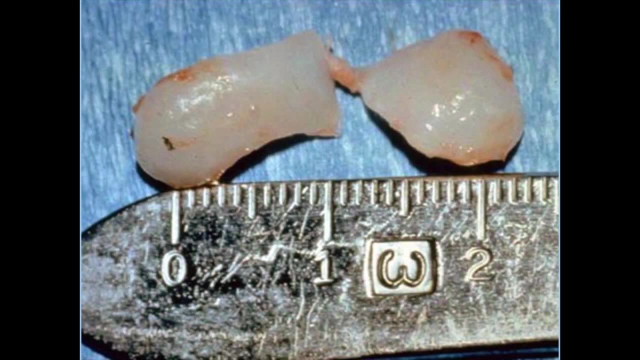 And here these are nude mice. Here we redid this guy's skull, Here this guy's cheek. If you open the animals up and look at them, it's pure white-glistening cartilage. Histologically it also looks like cartilage.